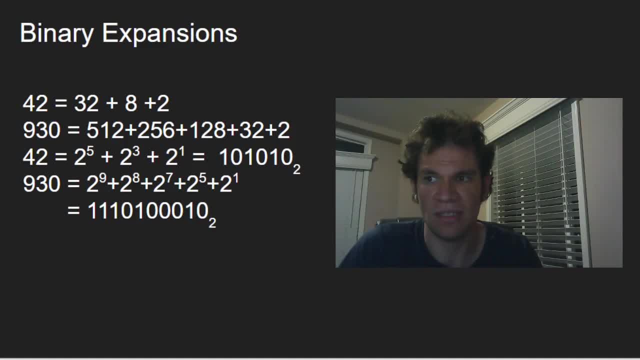 And, as you can see, if you check the binary binary expansion from right to left does once matches with the exponents on the tools over here, then a faster way to getting the binary expansion it could be going from bit by bit, first checking if the number is odd, or even then checking 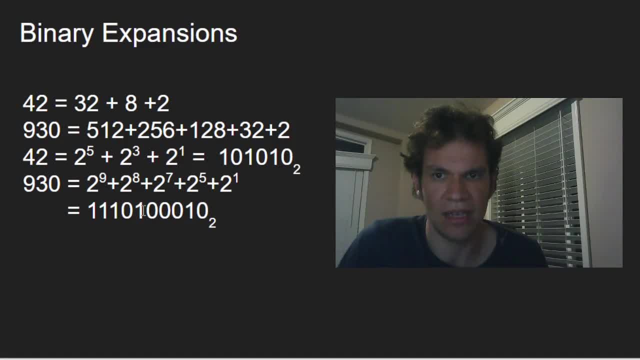 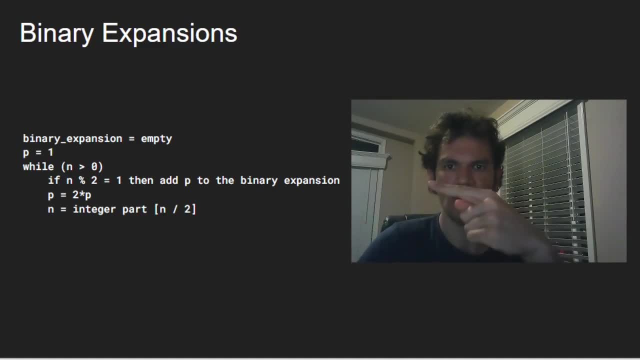 the next bit, then the next bit, and so on from right to left. summarizing: that could be the algorithm. also, many programming language had this trick over here that the smallest power of two that divides N can be found by using the this thing, And this runs in constant time. The languages with that are C++, Java or C. 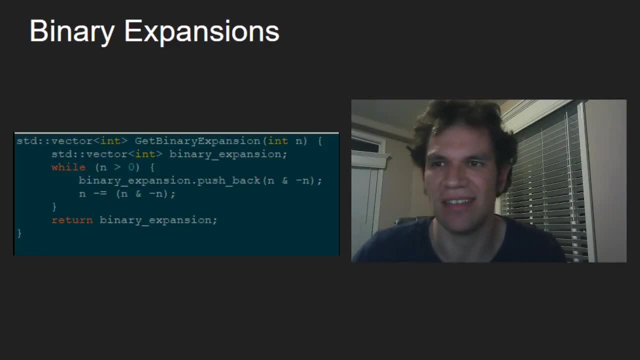 sharp. This property makes the implementation in C++ even simpler, As you can see. here it is, And here as well, And this could be useful for many things. The most straightforward that I could think about is the binary exponentiation, For example, if we want to know how much is. 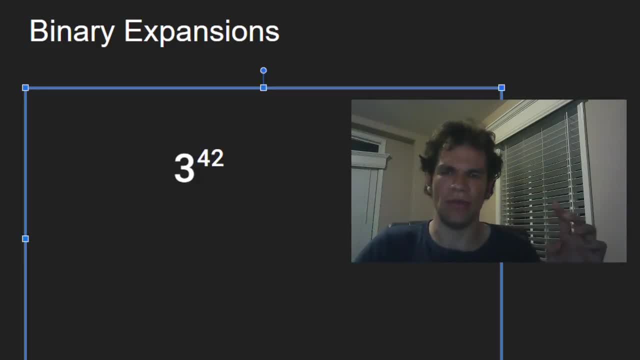 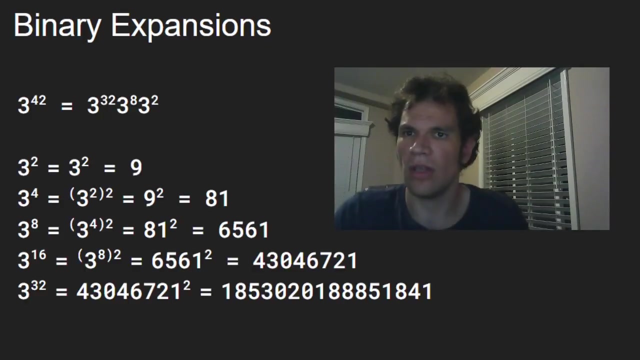 3 to the power of 42,. we don't need to multiply 3 by itself 42 times, Because we know that 42 equals 32 plus 8 plus 2.. So 3 to the power of 42. It's 3 to the power of 32 times 3 to the power of 8 times 3 to the power of 2.. We can square. 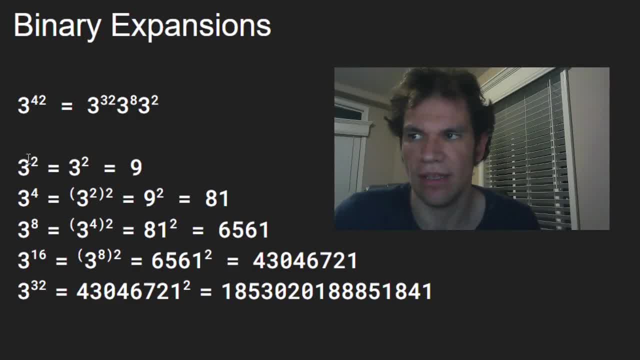 3 multiple times in order to get 3 to the power of 2,, 3 to the power of 4,, 3 to the power of 8,, 3 to the power of 16, and 3 to the power of 32.. 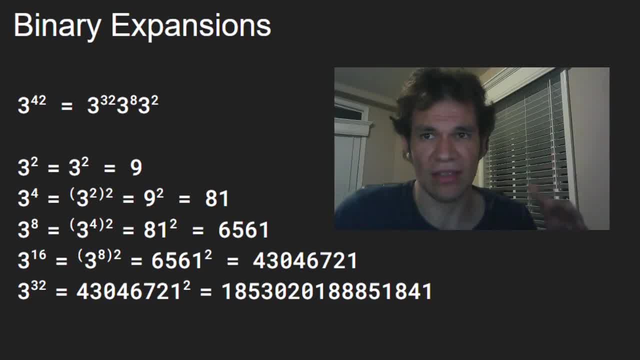 Each time we square the number it's only a single multiplication. So we raise it up: 3 to the power of 32, with only 1,, 2,, 3,, 4, and 5 multiplications. Then we know that 3 to the power of 42 is this thing over here And also we already. 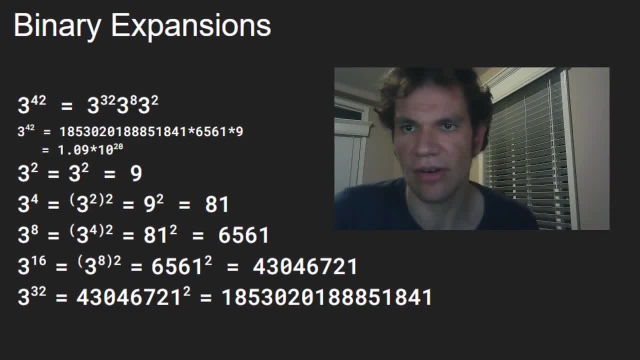 know the values of this. So 3 to the power of 42 equals 42 times 3 to the power of 6.. Then, after a simple substitution and a couple of multiplications, we get the result 1.09 times 10 to the power of 20.. 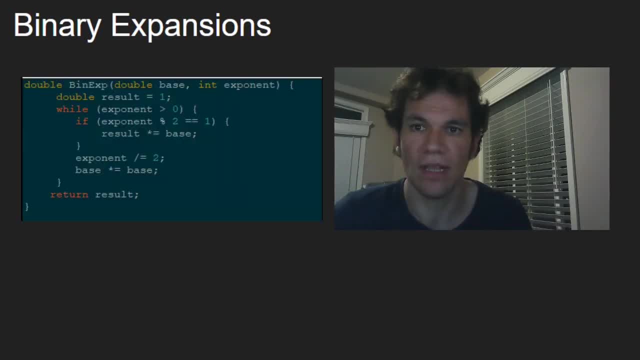 Of course, I know that you are here for the algorithms, So here is an implementation in C++. There is a recursive version of this same algorithm that is much easier to deduce and usually it's fast enough, But this iterative approach that I just showed you here. 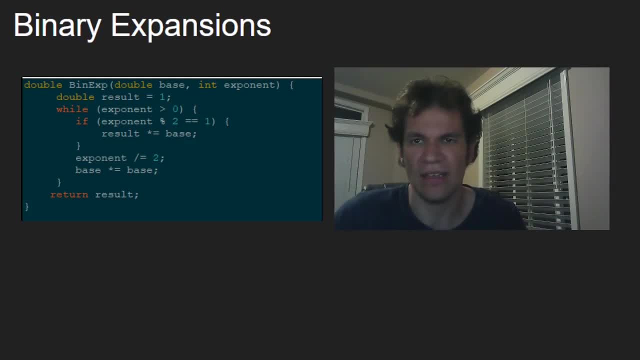 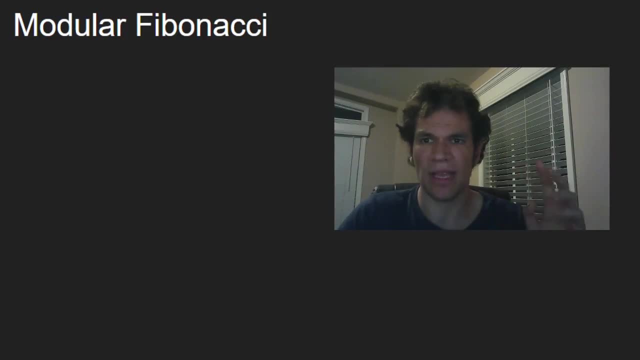 it will result more useful later in this same video, So I keep this iterative approach in mind. The next topic is the modular Fibonacci. As a quick recap, these are the Fibonacci numbers: Fibonacci of 0 is 0.. Fibonacci 1 is 1.. 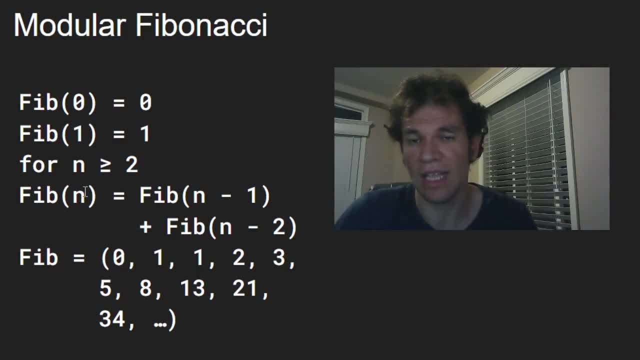 And after that each Fibonacci number is the sum of the previous two. So it starts with 0,, 1,, 1,, 2,, 3,, 5,, 8,, 13,, 21,, 34, and so on. 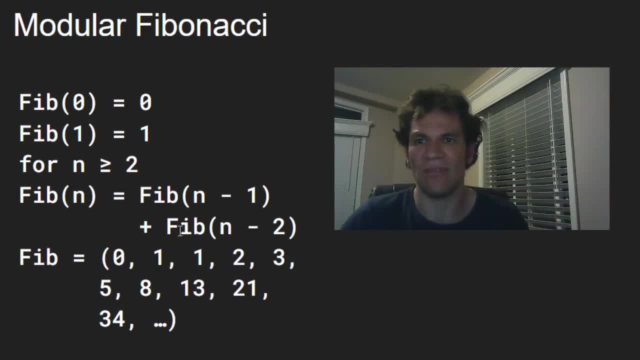 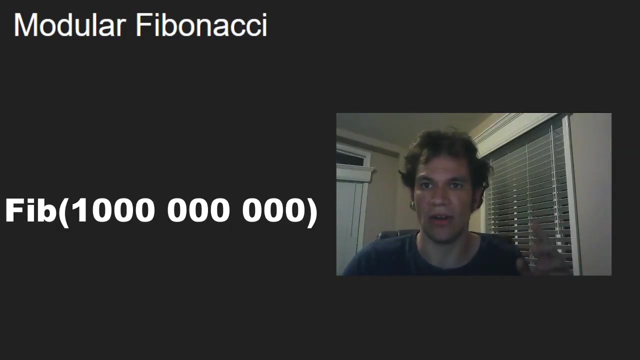 What we want to do is to find the fastest way to compute the last few digits of Fibonacci numbers. For example, if we want to find the last five digits or six digits of Fibonacci in millions, what would be a good algorithm for this? There are some ways to compute Fibonacci with that development. 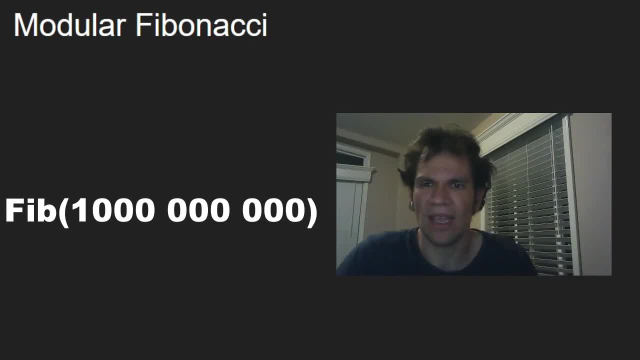 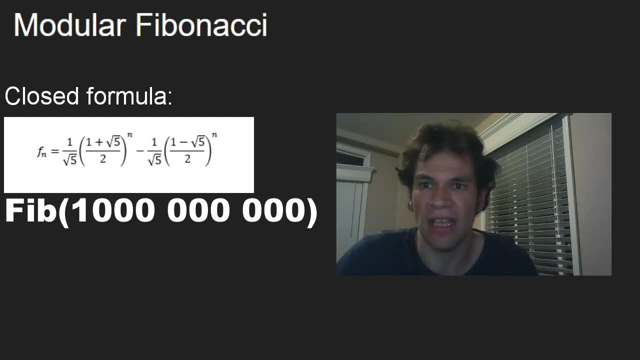 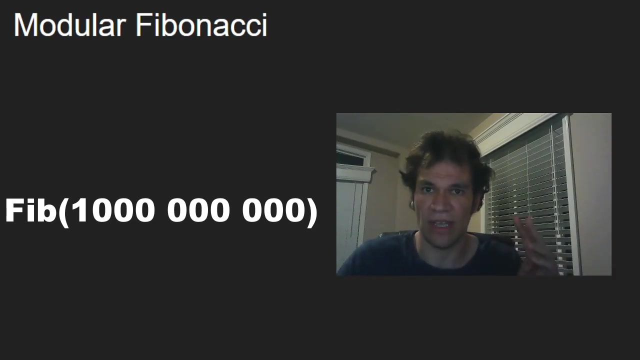 Fibonacci with a closed formula, but those ways are very impractical for this because it involves division and non-integer numbers, so it gets a lot of issues with precision. We want something that uses only integer numbers and no divisions of numbers. that could have 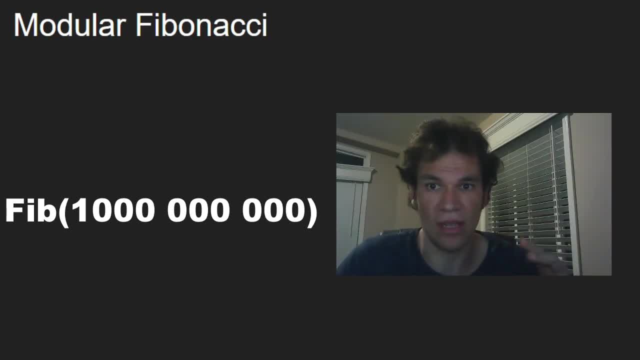 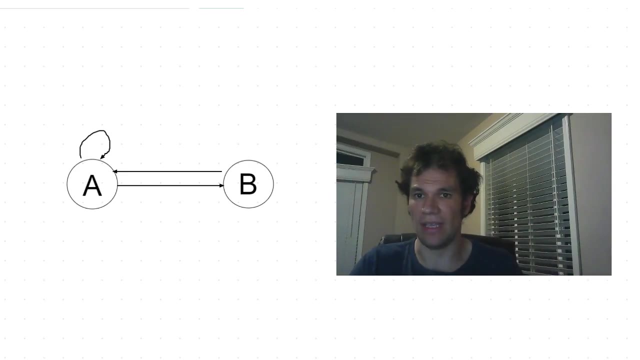 hundreds of digits, because Fibonacci numbers can have hundreds of digits. They grow very, very quickly. For finding a good algorithm, we will reformulate this problem in a different way. First, consider this graph over here. Suppose that we start on the node A. 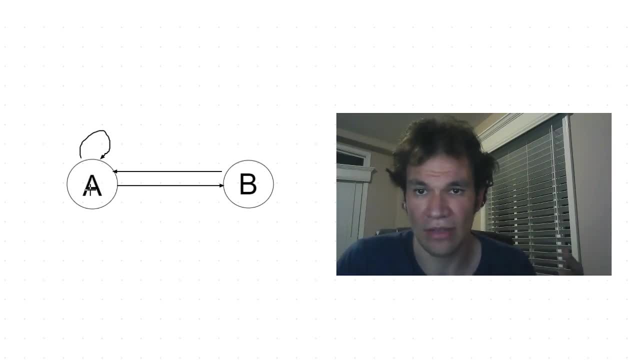 and now, in the same style we did with Bellman-Ford in the previous video, Let's count the number of paths to reach each node with zero steps. one step, two steps and so on. The way to compute that is: starting with zero steps. then there is only one path to reach the node A. 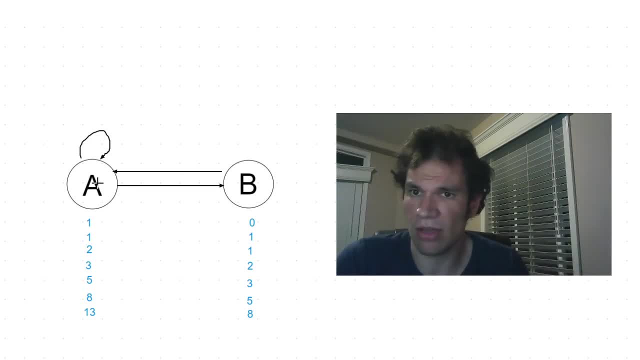 and there are no paths to reach the node B, because A is the starting node With one step. from A it can only go here or here. So it's one way to get to A and another way to get to B With two steps. it can reach A from A itself or from B. So 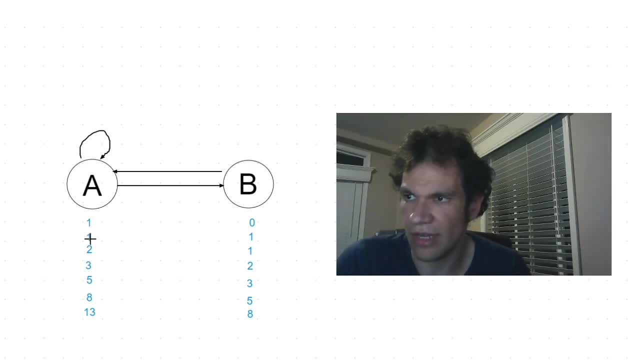 we just sum the two numbers over here and to get B with two steps it would need to get to A with one step. So we just copy this one from here to here. Then with three steps, again we check how many with two steps getting to A and getting to B, we add those two together and we get. 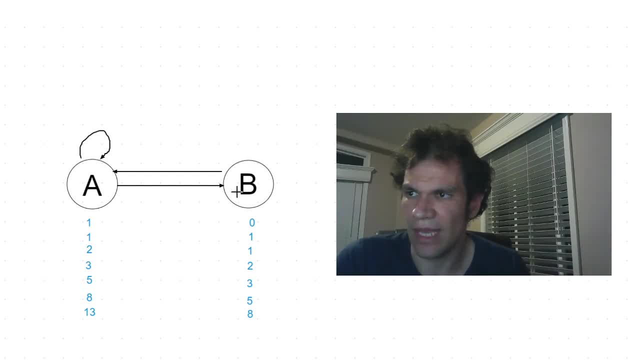 these three over here. and for B it can only come from A and we just copy the value from here. In general, for computing the number of paths to get to a certain node with certain number of steps, we just check which other nodes are pointing to that one and we sum the number of paths with one step less. In that way we 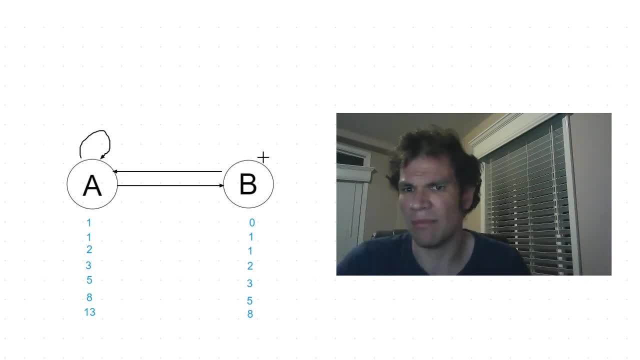 will check all the possibilities. but going back to the point, repeating this process until we get to here, I think you should have already seen the pattern. these ones are the Fibonacci numbers. It's not strange because for filling these numbers we are adding that these two together and these ones are just a copy. 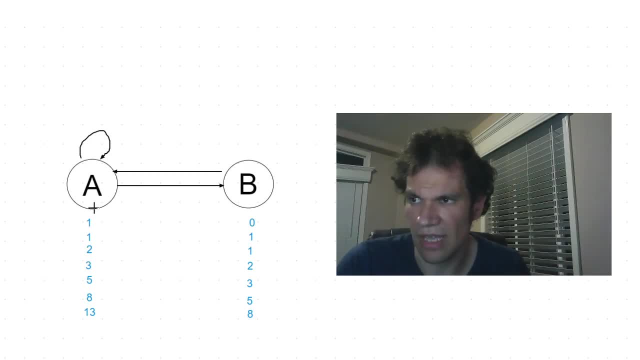 of the numbers over here, but shifted when you get to the other side of the board position downwards. Now we can reframe the problem of finding Fibonacci of n to find the number of paths from node A to node A with exactly n steps And 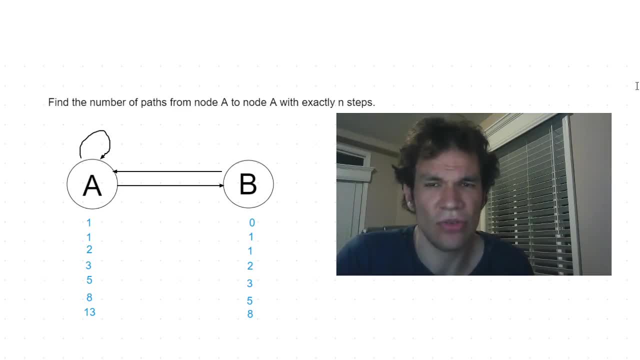 remember that we want to be able to choose a very big value for n, like a milliard, so we can't just compute n steps one by one. An advantage of reframing this problem as counting paths is that we have a lot of counting. 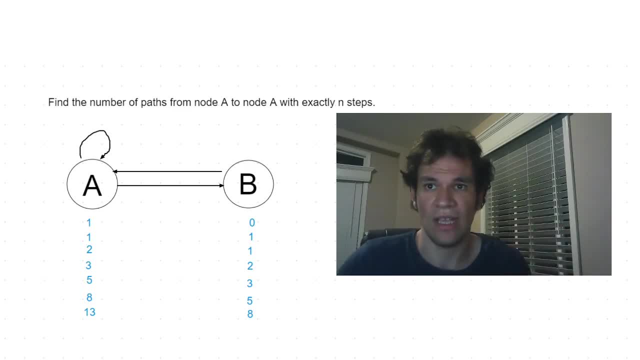 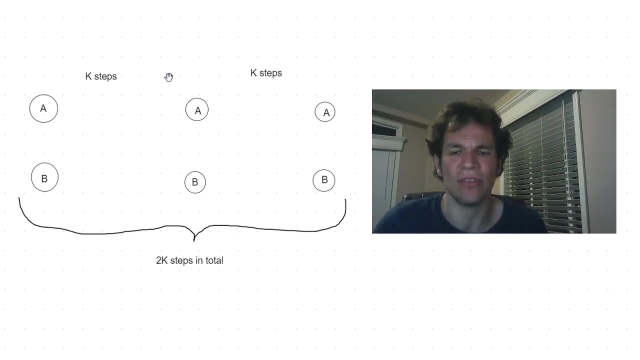 properties more grounded in our intuition. Instead of just dealing with some recurrences and algebraic jargon, we can rely more on problem-solving strategies that we can use to solve problems, Or what we call roughs or combinatorics. Our key observation to count the path is that, in order to take 2k, 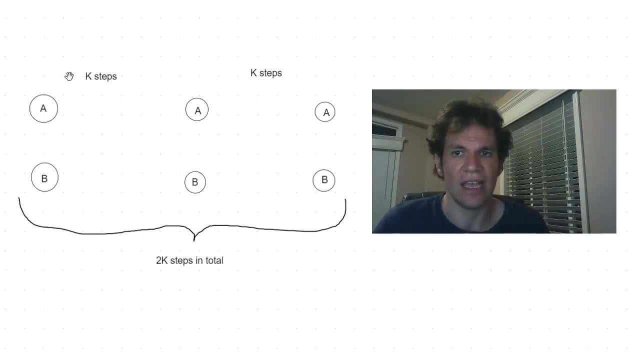 steps. we need to take k steps twice, So we can take k's from A to B and then k steps from B to A. to take k steps from A to B and then k steps from B to As. or we can start in A after k steps reach A and after another k steps reach A again. 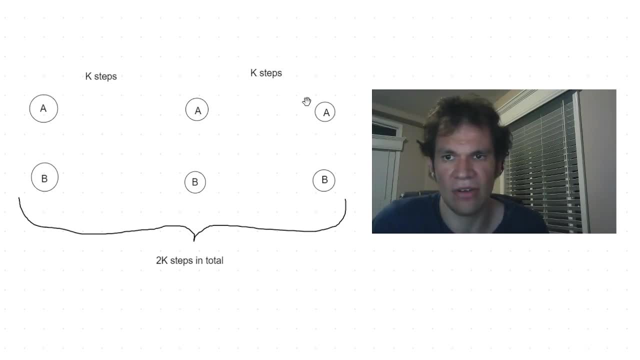 so, as you can see, in order to get from A to A, we can pass through these two different nodes in the middle. and now, in order to work with this in a more grounded way, let's define a function, and this function, p, is the number of paths from a node u to a node b, with exactly k steps. 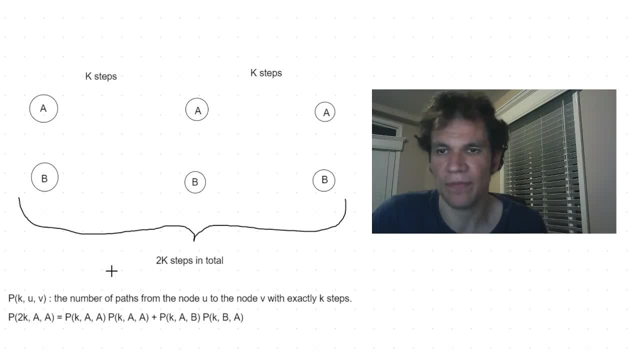 so with the previous reasoning we have that p from A to A. it's basically p of k from A to A times p of k from A to A, plus p of k from A to B times p of k of B to A. if you are struggling to get what this formula is, 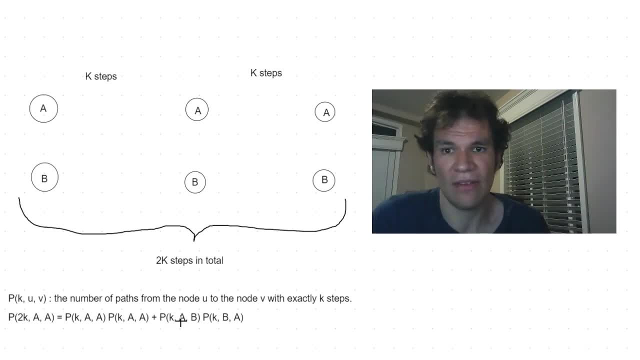 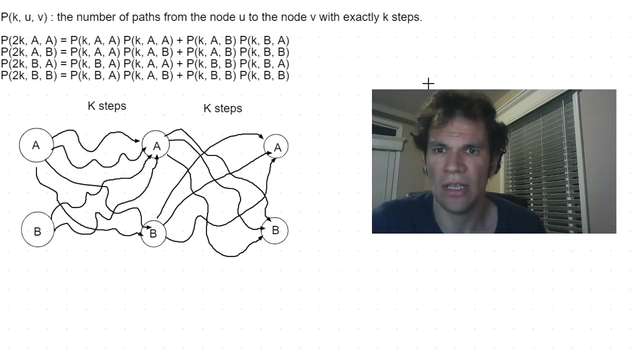 or why it is true. feel free to pause the video or to check my explanation again before continuing, because the next equation will use this and it will get more complicated. using a similar reasoning, it's possible to deduce these other three equations from going from from A to B. 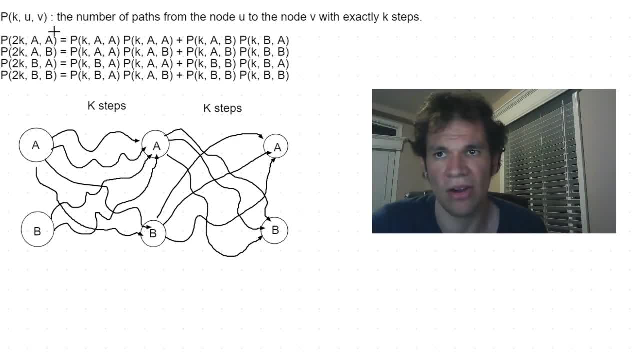 from B, ending in A or starting on B and ending on B. in all cases we need to start in the node, pass through an intermediate node in the middle and then get to the final node. these four equations combined are very powerful because if we know the value of p with k steps 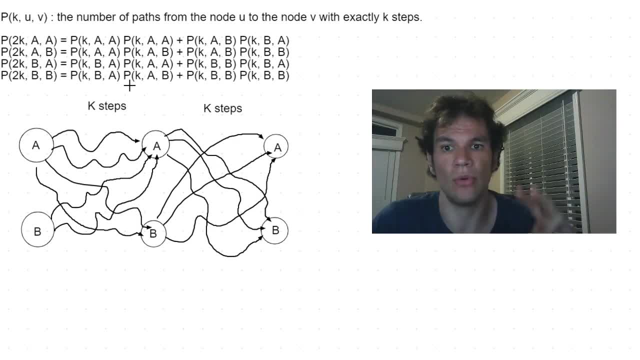 we can compute the value of p with 2k steps, only with eight multiplications. so, for example, if we know the value of k with a thousand steps, then we don't need to compute a thousand Fibonacci numbers to know how it could look like if we compute a thousand Fibonacci numbers. 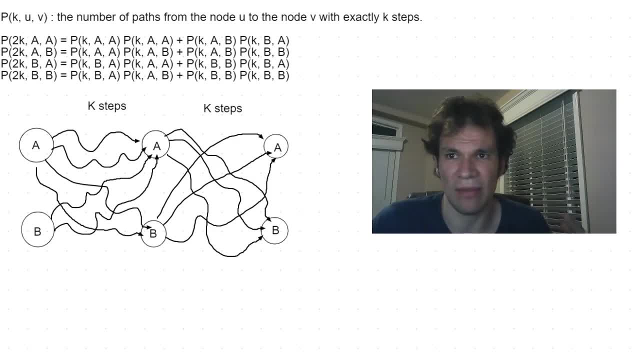 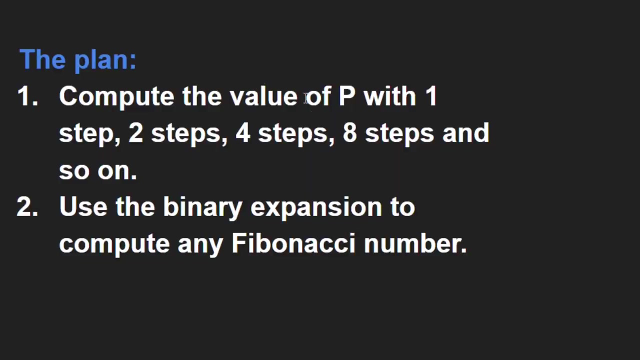 after another one thousand steps. the idea for solving this problem would be calculate the value of p with one step, with two steps, with four steps, eight steps and so on, and then we could use the binary expansion to know any Fibonacci numbers. so for the first step, let's define the matrix. 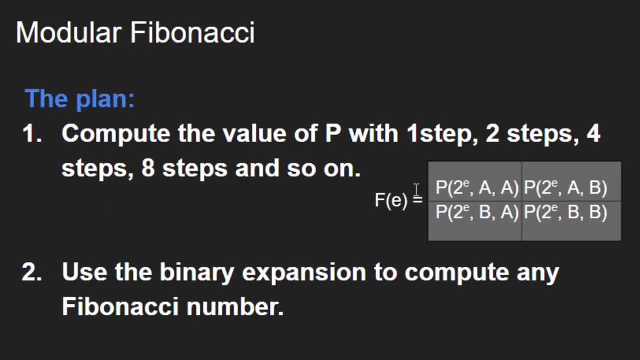 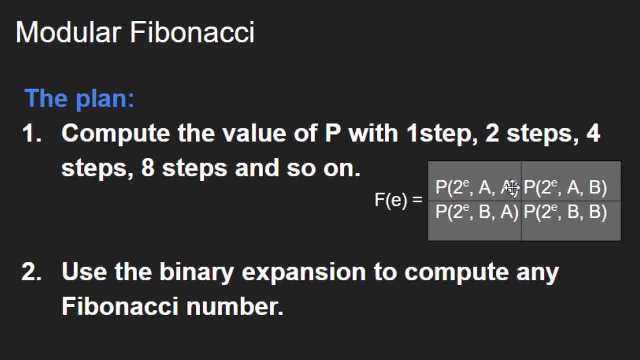 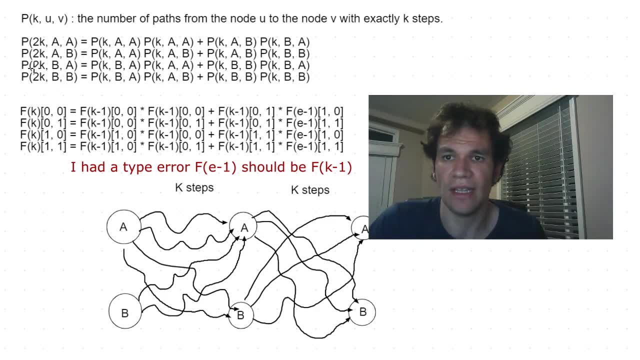 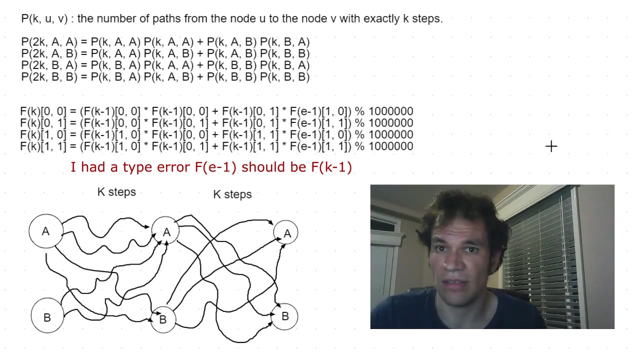 we aim to compute this using dynamic programming from these four properties that we deduced before. we can get these recurrences over here, and these recurrences allow us to compute the values of F using dynamic programming. and if we only want to know the last six digit, we could just add this thing over here. 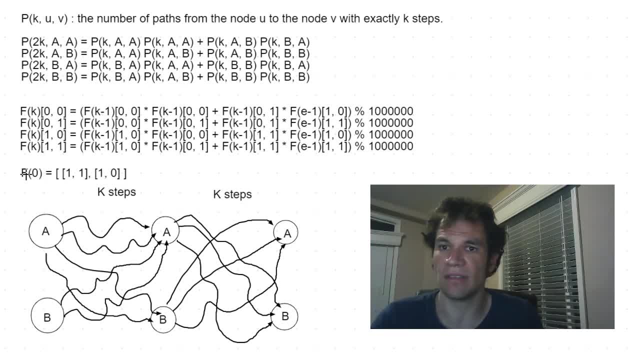 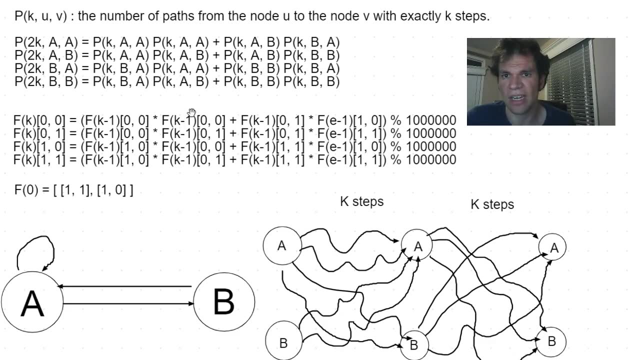 the base case of these recurrences would be basically the adjacency matrix of the graph. the base case of these recurrences would be basically the adjacency matrix of the graph. the base case of these recurrences would be basically the adjacency matrix of the graph. some of you may be thinking that this thing over here looks very, very similar. 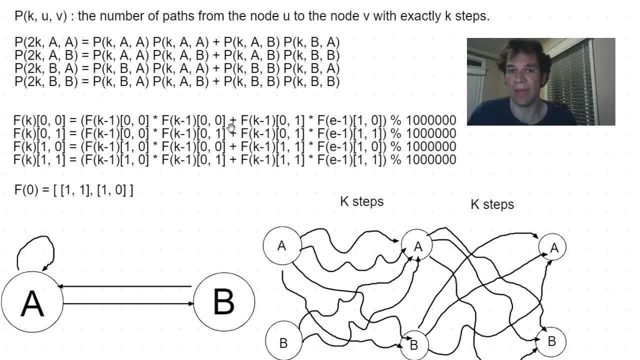 some of you may be thinking that this thing over here looks very, very similar, in fact identical, to matrix multiplication. actually, this is multiplying a matrix by itself, and yeah, that's totally right. however, I want you to stay in the dynamic programming, and yeah, that's totally right. however, I want you to stay in the dynamic programming. 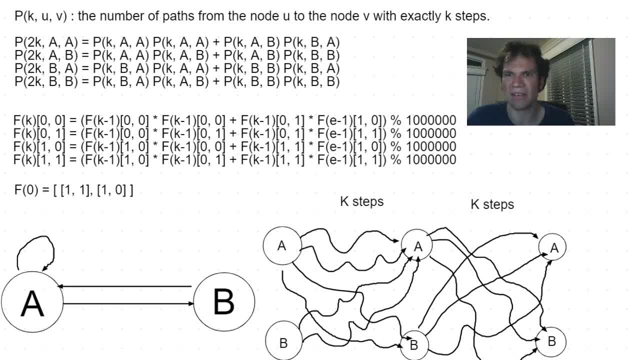 and yeah, that's totally right. however, I want you to stay in the dynamic programming point of view point of view point of view, because this math mindset of computing, a because this math mindset of computing, a because this math mindset of computing a table using power of two is very useful. 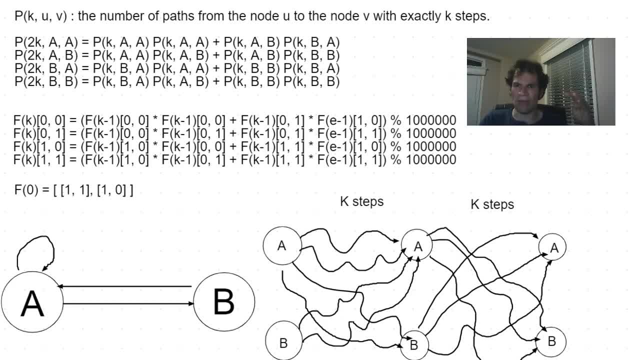 table using power of two is very useful. table using power of two is very useful for many other problems that we will be, for many other problems that we will be, for many other problems that we will be checking out in this video as well. if we checking out in this video as well, if we 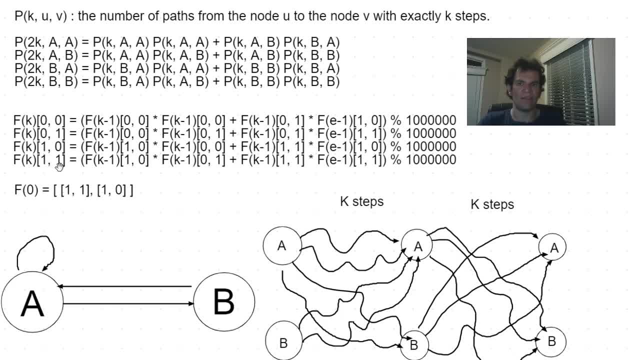 checking out in this video as well. if we compute all the values of compute all the values of compute, all the values of f up to 31, f up to 31, f up to 31, then we could compute fit for any, then we could compute fit for any. 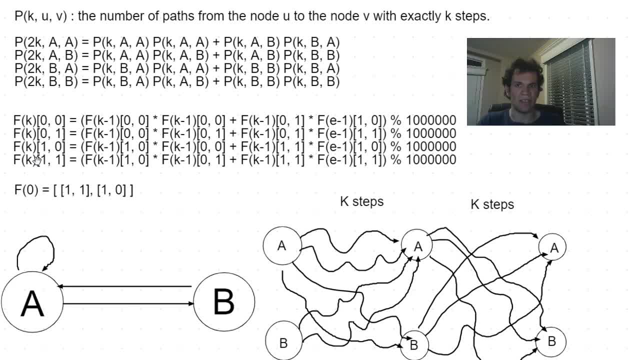 then we could compute fit for any power, power power of 2 that fits in a 32-bit input. We said before the goal is first to compute the values for the power of 2 and then extend it for all the other numbers. We already know how. 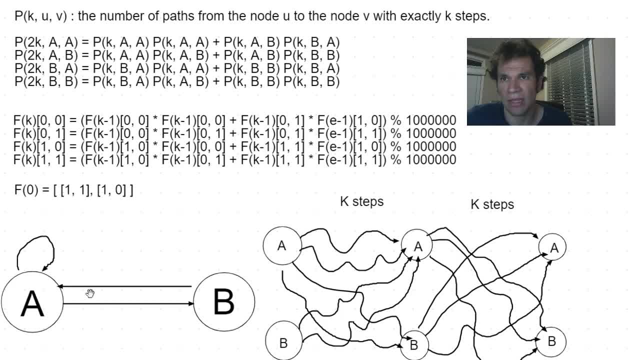 to achieve the first step. but now, going back to the graph, if we know the number of ways to reach A with n steps and the number of ways to reach B with n steps, we could advance 2k steps with this simple algorithm. 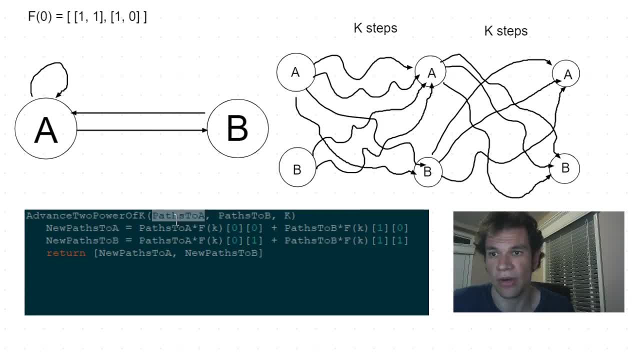 This. This algorithm takes the number of paths to reach the node A and the number of paths to reach the node B with n steps and returns the number of paths to reach A and to reach B with n plus 2 to the power of k steps. 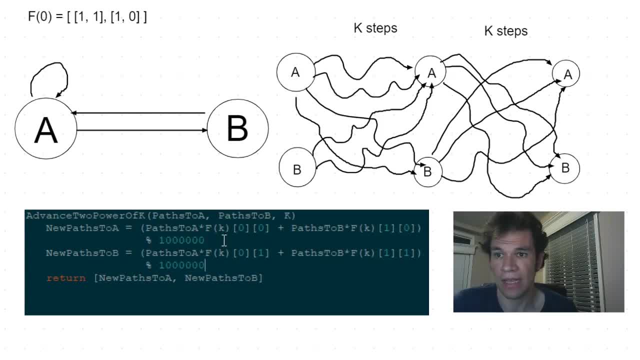 and if we are computing the last six digits instead of the whole numbers, then it is enough to just add this thing. Now, knowing how to advance any power of two steps, we will use the same idea of a binary exponentiation algorithm that looks like the one we used in the pre- اب Pandora. 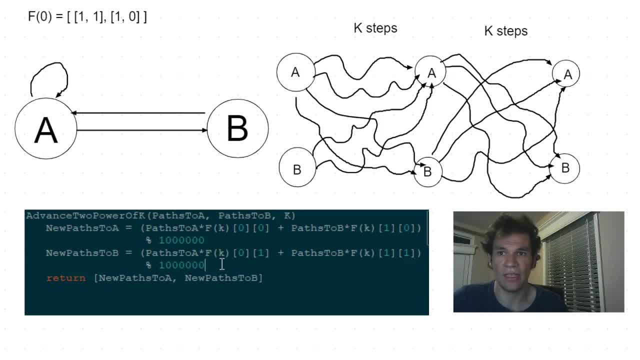 It is a pointer- over the number series and then the 로 take the arrow shape. The problem of omitting posição is because the output of the Pea of is川 othercha goes to L. in the exponentiation algorithm that looks like A that we discussed before to compute the Fibonacci number, this time. 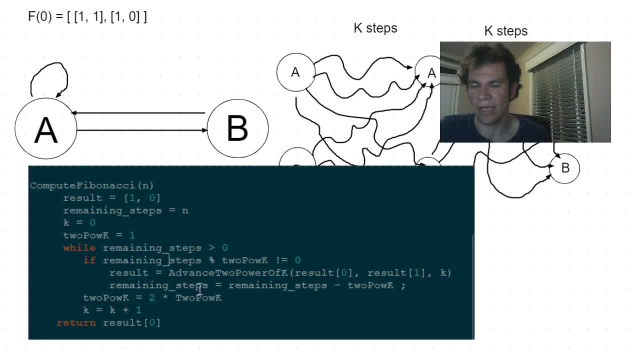 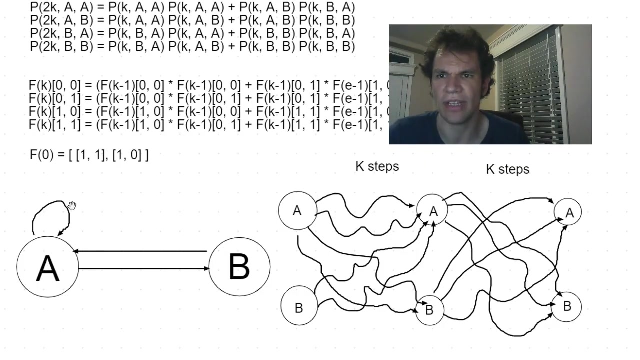 As you can see, it's the same idea than binary exponentiation: going from the right to left, checking which bits are powered on and then advancing the corresponding number of steps. Something important to notice is that if we use a different graph than the one that is, 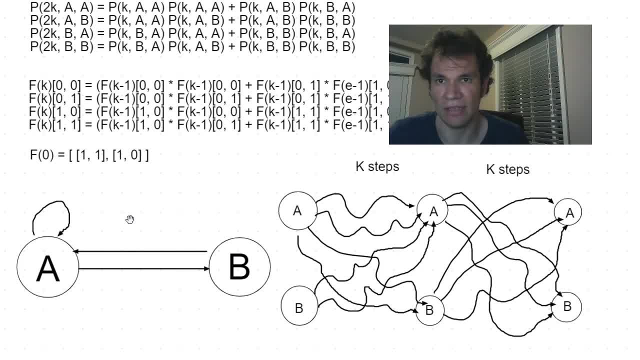 here, but we still count the paths in the same way, using dynamic programming and grouping on powers of 2, and with the binary expansion all of this, we could compute a big variety of functions depending on the graph we choose. For example, we could compute the first columns of any row of the Pascal triangle.